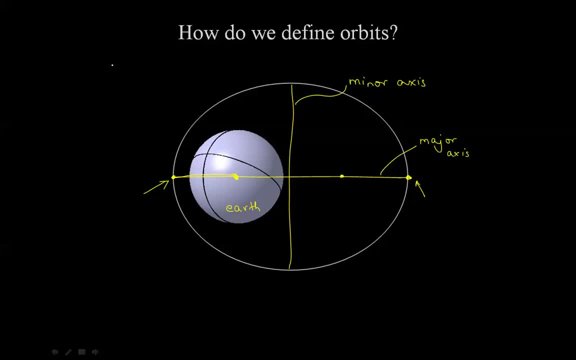 points or locations in that orbit. These two points together are known as the absciss, This one here being the periapsis and this one here being the apoapsis: Apo for furthest, and peri for closest or nearest. Here we can see that if I were to change the size of the 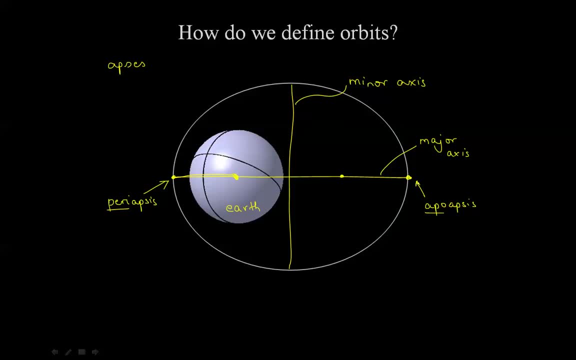 major axis and make it longer and longer and longer, the orbit would drastically increase in size. And that is our first parameter: size, And the size is indicated by the length of half the major axis, also known as the semi-major axis, Semi-major axis, And that is our first parameter denoted by the letter A. 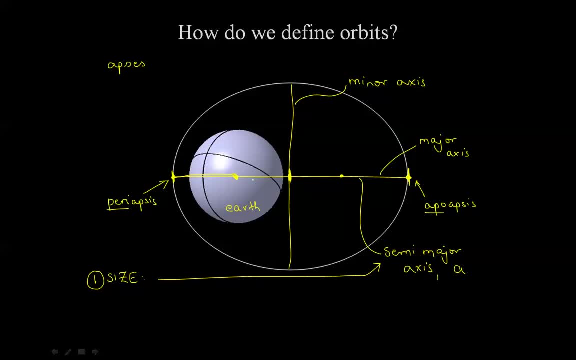 Now notice that if I hold the major axis length steady there and if I were to change the length of the minor axis so that it gets shorter, for example, the orbit will flatten out. Now if I change the length of the minor axis to make it longer, there will come a point. 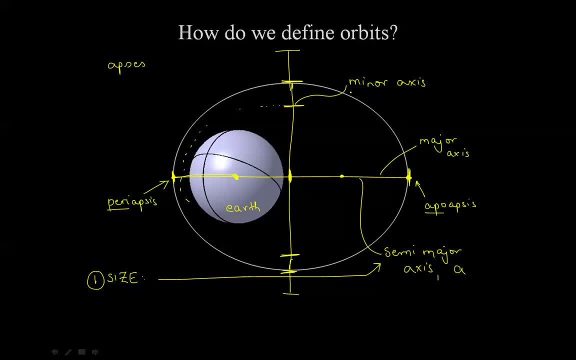 where the minor axis length is equal to the major axis length and the orbit will therefore be perfectly circular. This is our second element, Because the minor axis length determines how eccentric the orbit is. the second element that determines the shape of the orbit is called eccentricity. 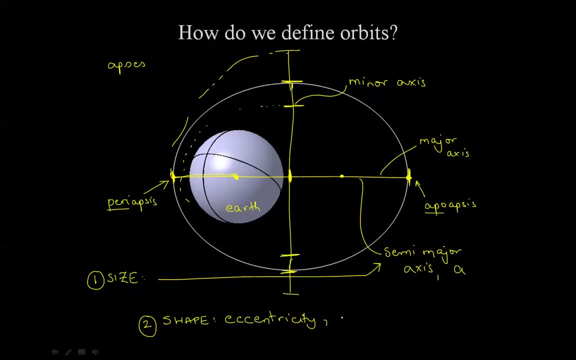 The second element that determines the shape of the orbit is called eccentricity, and it is directly related to the radius of the periapsis, the distance from the center of the Earth to the periapsis. the radius of the apoapsis, the distance from the center. 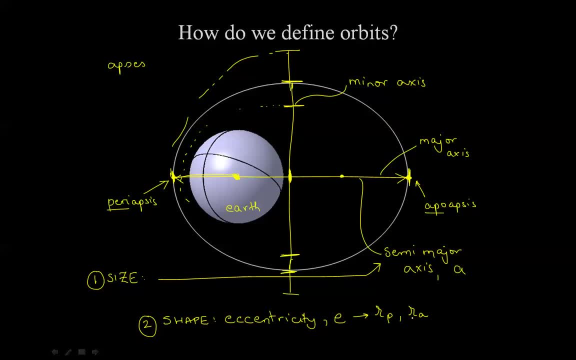 to the apoapsis, and because the radius of the periapsis plus the radius of the apoapsis equals the total length of the major axis, It also depends on the length of the major axis a. We have defined the size and the shape. Now we need to understand how this orbit is oriented. 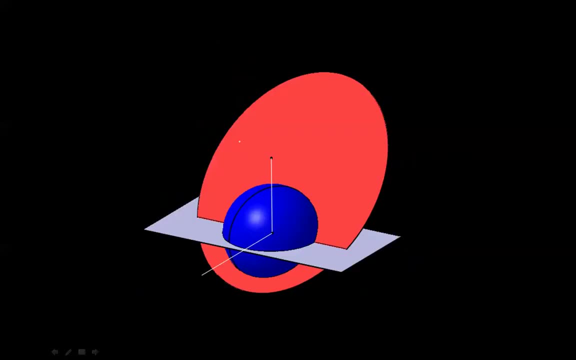 around the Earth. In this image I have drawn it in 3D format. It can be a little tricky because I am depicting a 3D orbit or a 3D concept on basically a 2D screen, But here we see the blue Earth. 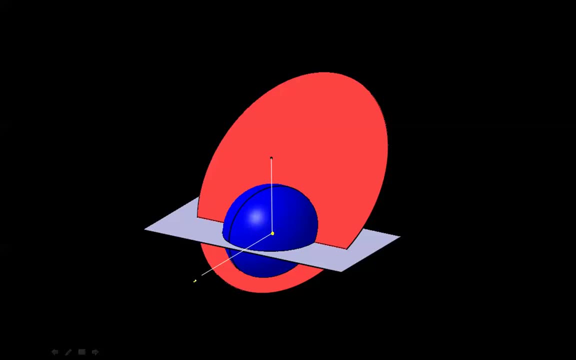 The center of the Earth has two axes going through it: One here, or actually let's start with this one. one here that goes through the north and the south poles, the north-south pole axis, or the axis of the poles, and this one here, which is seemingly arbitrary axis. 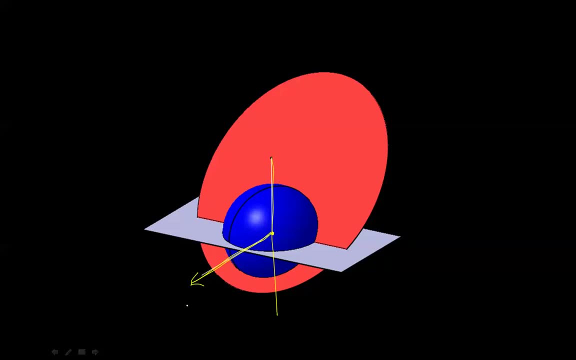 because it is an arbitrary axis and it points to the vernal equinox. Vernal equinox, The gray plane here, is the one that passes through the equator of the Earth and is known as the equatorial plane. Equatorial plane. Similarly, the orbit also passes through its 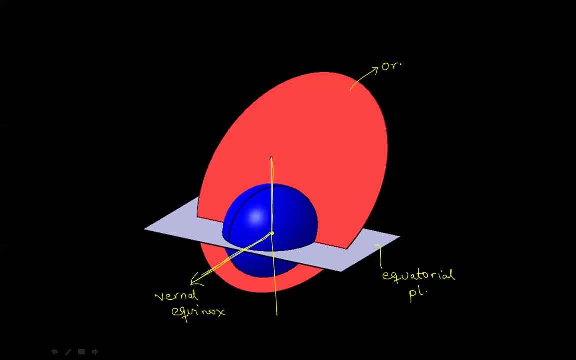 own plane, the red one, known as the orbital plane. Notice here that the orbital plane intersects the equatorial plane, forming a line of intersection where there are two points where an object going this way across this point here, will tend to cross the equatorial plane, ascending it, ascending from below to 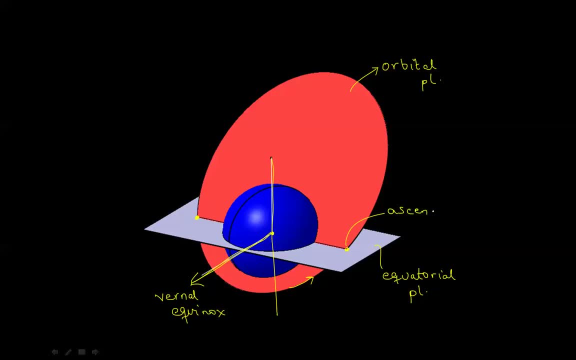 above it. This point is known, therefore, as the ascending node. Similarly, on the other side, the object will descend to below the equatorial plane, and this point, therefore, is known as the descending node. If here I hold the Earth and equatorial plane and the north-south pole axis steady, or the 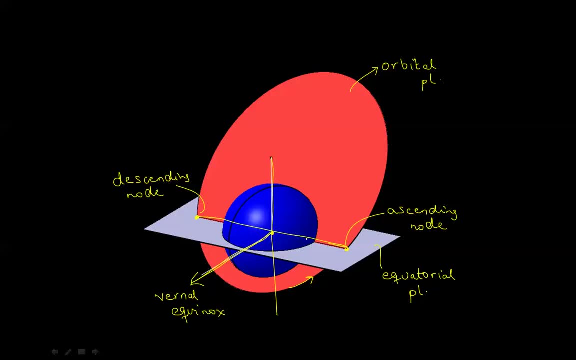 north-south pole axis steady and the line that joins the two nodes steady. what I can do is I can change the tilt of this orbit, around this line that intersects the two nodes, either by tilting it this way or rotating it this way, or 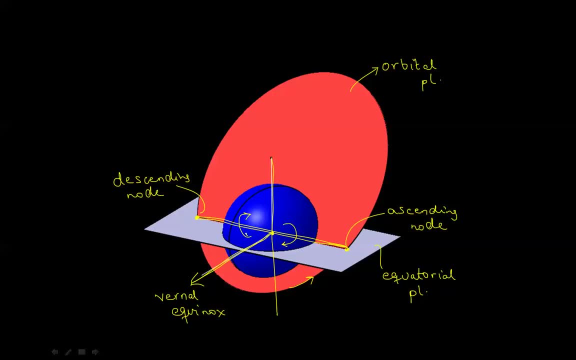 rotating it the other way or this way. This determines the angle between the orbital plane and the equatorial plane. That angle there, And that is our third parameter, that which determines the tilt of the orbit. The parameter itself is known as the tilt of the equatorial. 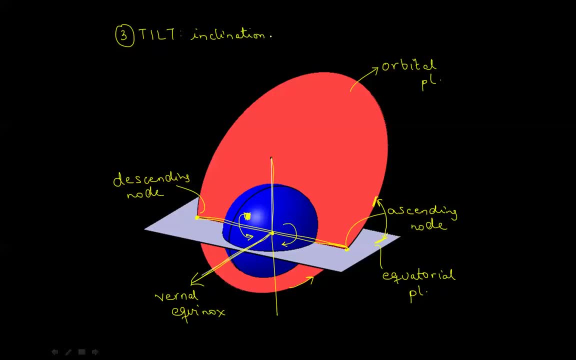 plane Inclination denoted by the letter. I measured in degrees from the equatorial plane to the orbital plane. Notice here that there is another angle. If I hold the Earth and the equatorial plane, as well as the north-south pole axis, steady, I can, without changing this tilt. 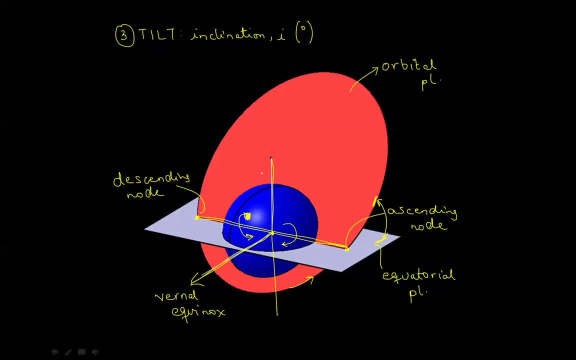 angle. I can simply swivel this orbit around the north-south pole. I can keep on tilting the pole one way or the other way, thereby shifting both the nodes this way or that way, depending on how I or swivel this orbit. And this is the fourth. 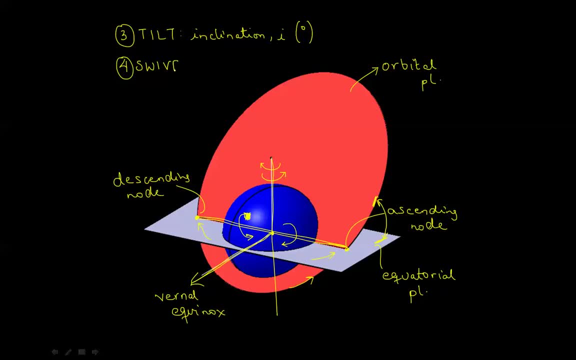 parameter, that which determines the swivel of the orbit. How do we measure it? Notice that the swivel changes this angle from the vernal equinox to the ascending node. That angle there, That angle is known as the longitude of the ascending node. 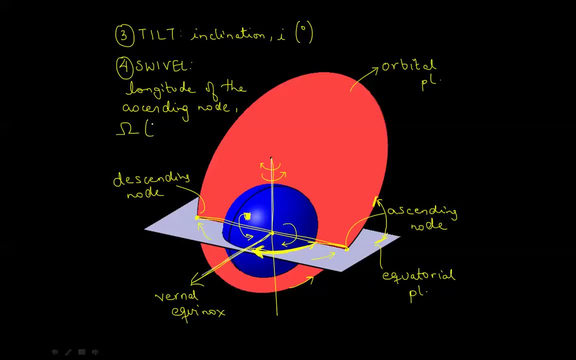 It is denoted by the capital Greek letter, omega, measured in degrees along the equatorial plane, from the vernal equinox to the ascending node. We have determined the size and the shape, as well as the orientation. So we have completely determined the orbit itself. but if there is an object in this orbit, 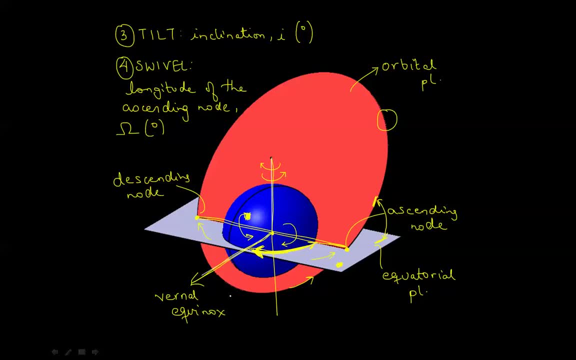 we still haven't figured out how to position it and how to locate it. We'll do that now. Notice in this cleaner picture again, The two nodes, and this looks like it would be the periapsis: the closest point of closest approach, and similarly that one over there will be the point of furthest approach. 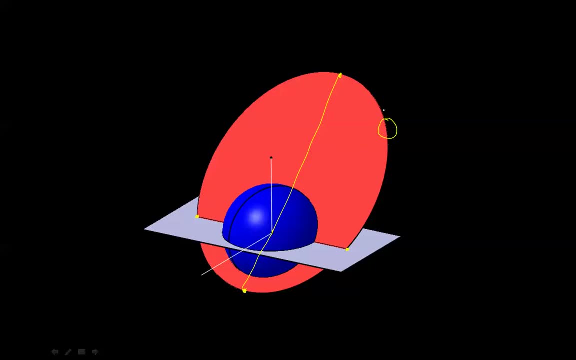 Suppose that there is an object in this orbit, at this location, going this way, It is approaching the apoapsis and has already passed the periapsis. But where is the periapsis in the orbit? Well, let's see, I can hold everything steady, including the nodes and the equatorial plane and the inclination. 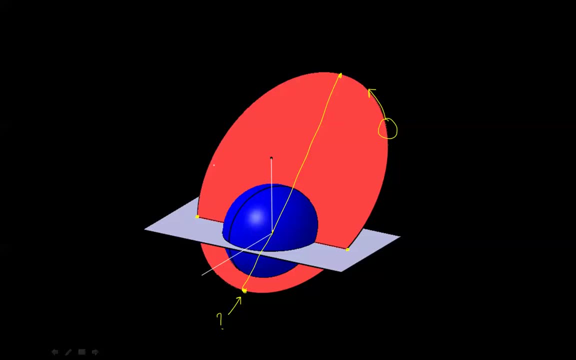 and I can change the length and the width of the orbit to determine where this periapsis lies. It could basically lie here Or say here. Suppose that it lies here, Okay, Cool, Nice Cool. in the orbital plane from the line that joins the ascending node. 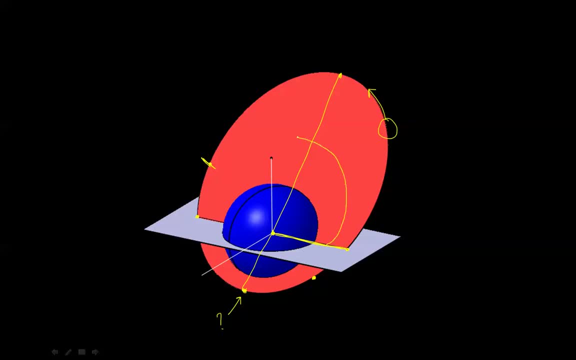 to the center of the Earth, all the way to the line that joins the periapsis, to the center of the Earth. That angle there, That angle is our fifth element and this determines the location of the periapsis. The location and the nomenclature is the argument of 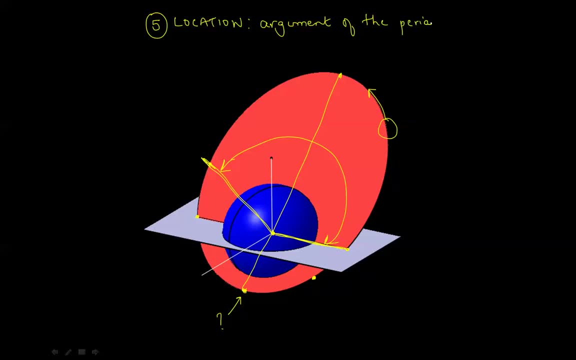 the periapsis, and it is denoted by the letter omega in its lowercase form, measured in degrees, this time in the orbital plane, not in the equatorial plane, from the line of the ascending node to the periapsis radius, always in a counterclockwise direction. 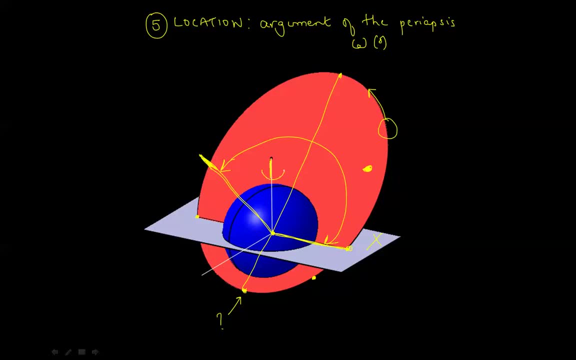 when measured from the North Pole, so counterclockwise. that way, as you can see, Now we have determined where the location of the periapsis is, but where is the location of the body, that is, where is the body positioned in this orbit? Notice that, if suppose, if this is the periapsis. so 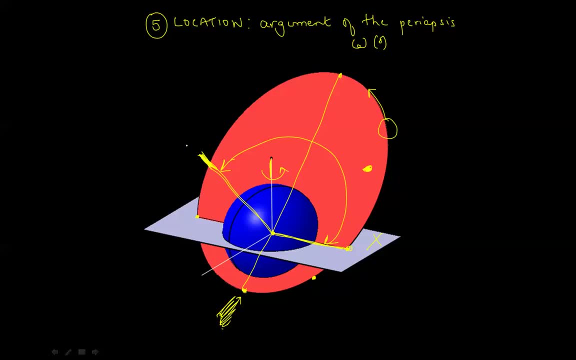 we'll erase that point. suppose that this is the periapsis here denoted by the asterisk. Now the body has crossed the periapsis and it also forms an angle from the line of the periapsis or the radius of the periapsis. 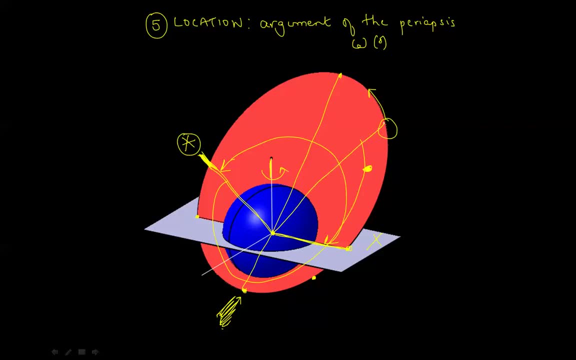 to the line that joins the center of the body to the center of the Earth itself. That is this angle there, And this is our sixth element, the position of the object in the orbit itself. and this angle is known as true anomaly denoted by the letter. 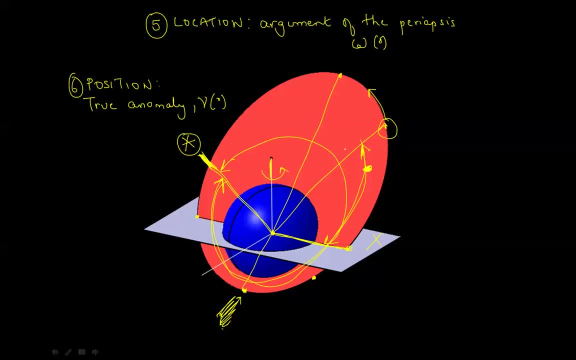 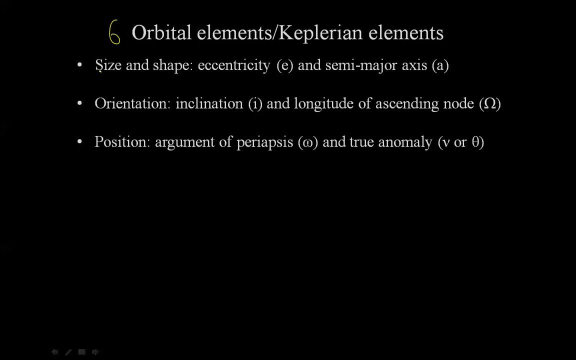 mu, again measured in degrees, again in the orbital plane, from the line or the radius of the periapsis, counterclockwise in the orbital plane, To actually where the body is positioned. So we have determined the six orbital classical or caplerian elements. size and shape of the orbit are given respectively by the. 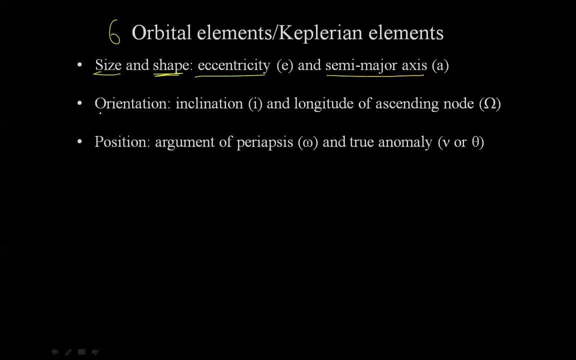 semi-major axis and the eccentricity. The orientation of the orbit in space is given by the tilt of the orbit, determined by the inclination and the swivel of the orbit. The position of the periapsis is determined by the inclination and the swivel of the orbit. 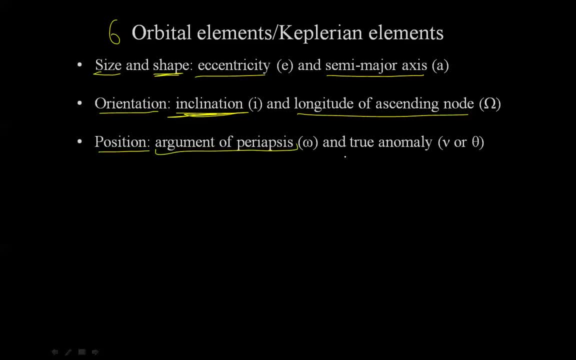 is given by the argument of the periapsis and the location of the body from the periapsis is given by the true anomaly. in this way we can hold any of the six elements steady and change any of the other elements and we have entirely different orbits. yet we can define all orbits using just 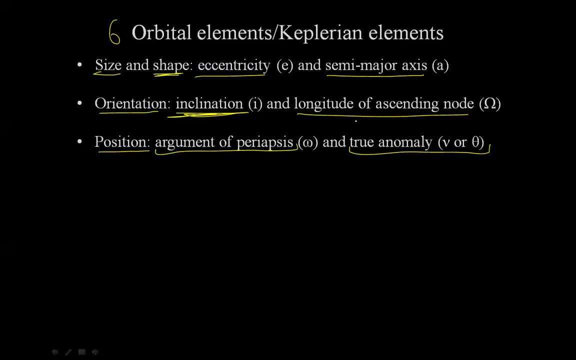 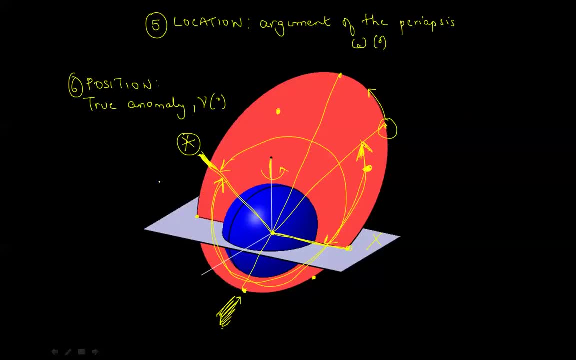 these six elements. however, as you will see, there are some special cases. for example, if I go back- actually let me go back to a clean picture- if I have the periapsis here and the apoapsis here, and if I reduce or increase the length of the minor axis so that the orbit becomes, let's say, 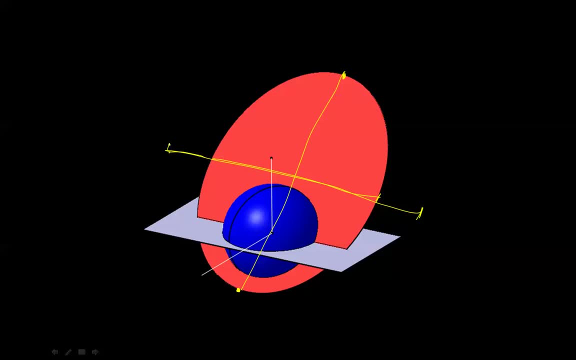 this is the increased length of the orbit of the minor axis, such that the orbit is perfectly circular. In a circular orbit there is no point that is any further away than any other point. They're all at the same distance from the center of the orbit. So in this case,